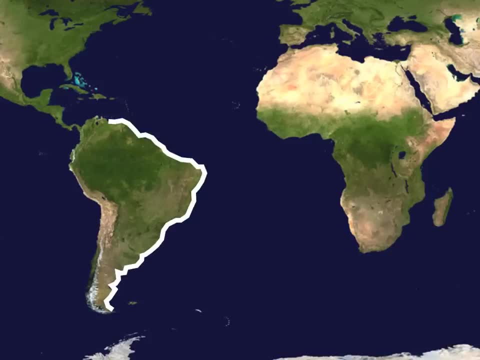 at certain parts of the world, like the eastern coast of South America and the west coast of Africa, for example, they look like they belong together. Now I hate to break your hearts, but this is not a groundbreaking discovery. In fact, people have known this for hundreds of years. 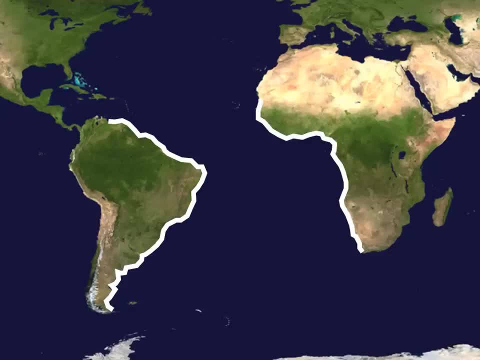 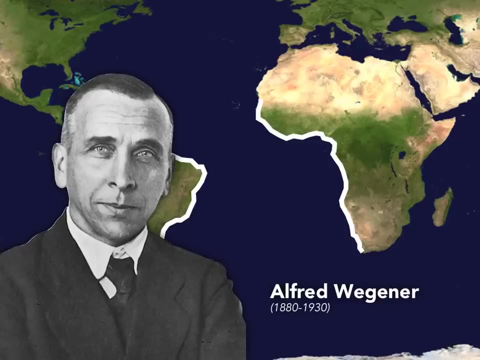 Most people have just taken it for granted that that's just the way the continents look, But there have been a few brave scientists throughout history who have thought that it must be something more. Let me introduce you to one. This is Alfred Wegener. Alfred Wegener was a German meteorologist. He studied weather. He 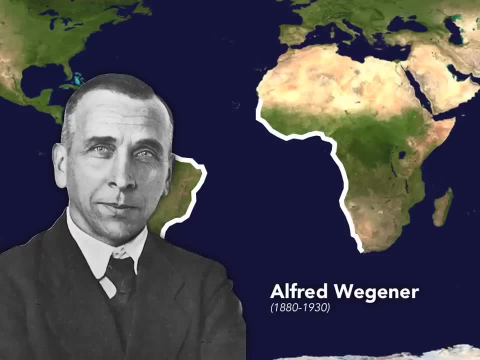 lived in the late 1800s and early 1900s, And as a weather person, a scientist of the atmosphere, of course- Wegener spent a lot of time looking at maps, And so he noticed this strange shape phenomenon. He was able to get past it. He actually devoted his whole life to it. He came up with a radical 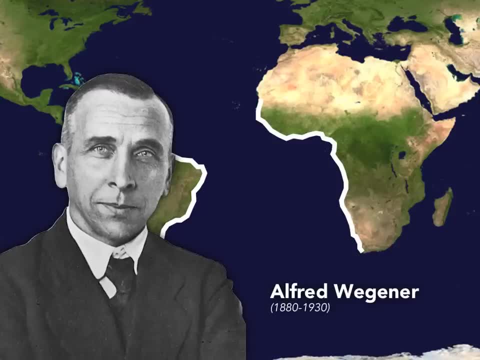 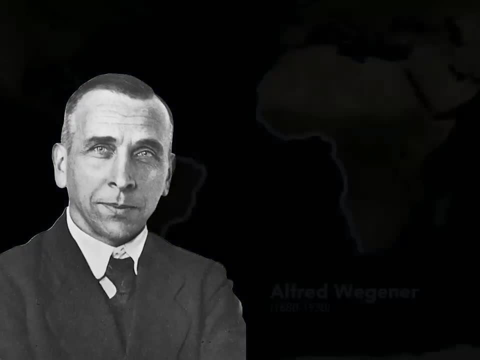 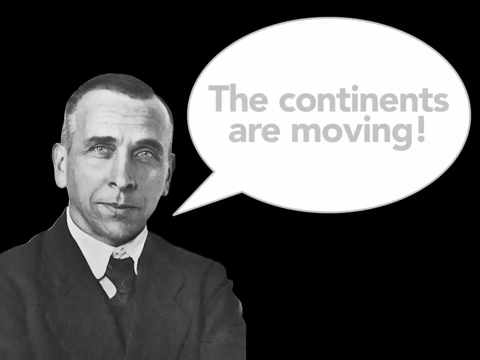 theory that suggested that the continents were actually once connected and then somehow ripped apart to where they are today. He came out and said: I think the continents are moving. Of course people thought this was a silly thought to have. How could a continent possibly? 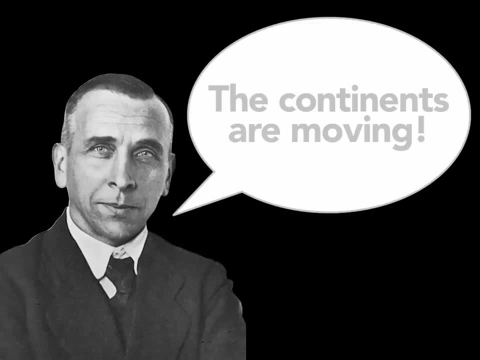 move, And Wegener really thought that this was the case, And so he devoted his whole career to studying this and coming up with proof of this radical idea. In fact, Wegener didn't just think the continents were moving, He actually believed that there was a time when they were all connected. 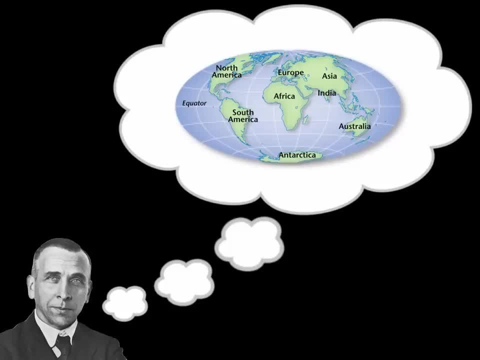 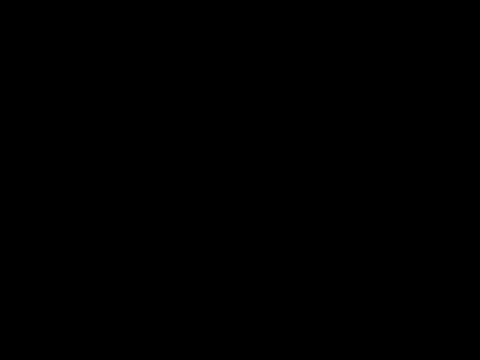 and they have since drifted apart to their current locations. He even came up with a name for that supercontinent that existed in the past. He called it Pangea, the supercontinent that he believed existed about 200 years ago. He called it Pangea. He called it Pangea. He called it Pangea. 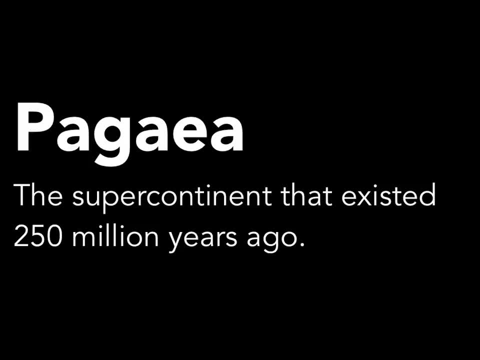 Pangea or Pangea was actually an appropriate name. It's a Greek term that means entire Earth or all Earth. So if you think about it, when all the continents were together, if Wegener is correct, it would make sense to call that landmass Pangea. 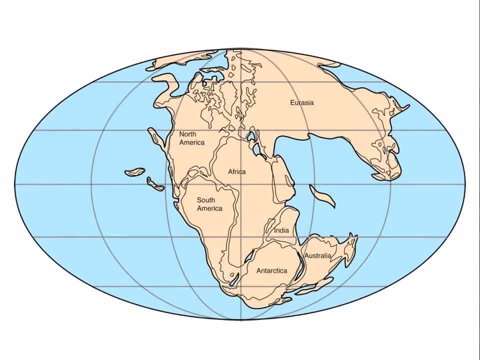 Here's what we geh thought it looked like. You can see within this diagram the modern day continents of North America, Africa, South America, Antarctica, India, etc. But they don't look quite the same way they do today and of course they're in totally. 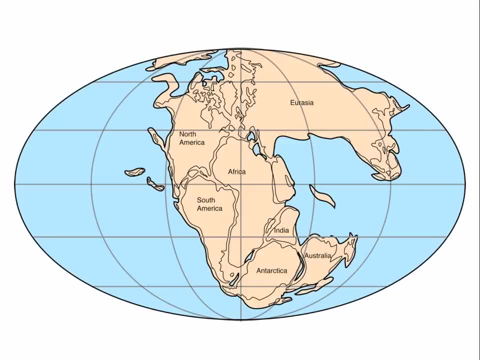 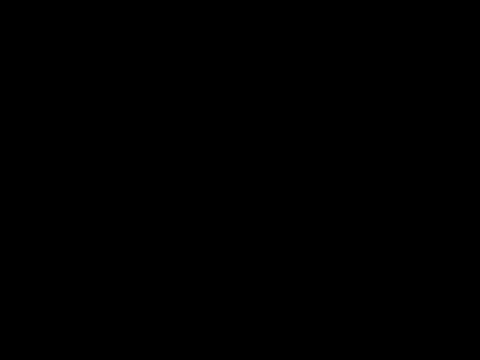 different positions all connected into this one supercontinent. Now, people thought Wegener was a little bit nutty, and so he knew that if he was going to make any headway with this idea, he had to come up with evidence, And so we're going to take a look. 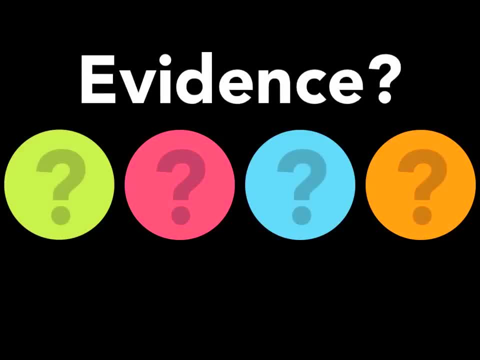 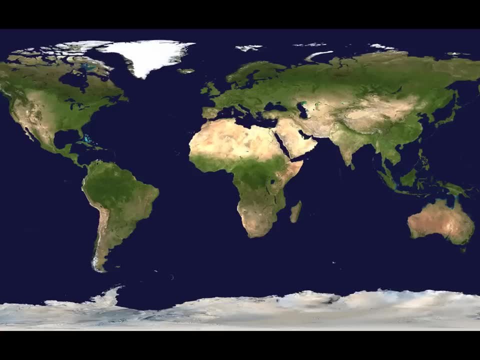 at four pieces of evidence that Wegener put together to prove to the public that the continents had in fact drifted. Let's take a look at his first piece of evidence. We'll go back to this map here Now. the first piece of evidence we've actually already discussed. It's simply. 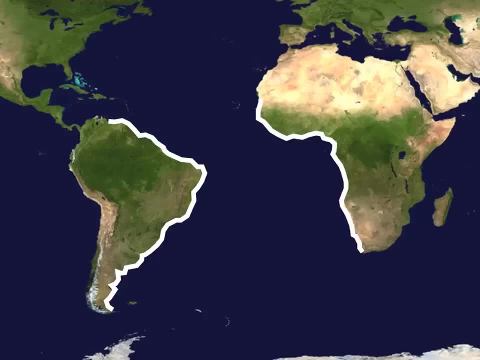 the observation that the continents appear to fit together- As simple as that. Wegener didn't believe that this could be simply a coincidence. He feels like there's no possible way the continents would have this appearance just randomly, And so this becomes evidence number one. 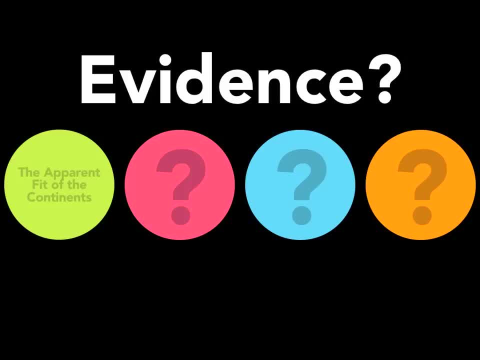 We will call it the apparent fit of the continents, the fact that they look like they fit together, And just to expand on that a little bit: essentially the coastlines of the continents appear to fit together, kind of like the pieces of a puzzle. But 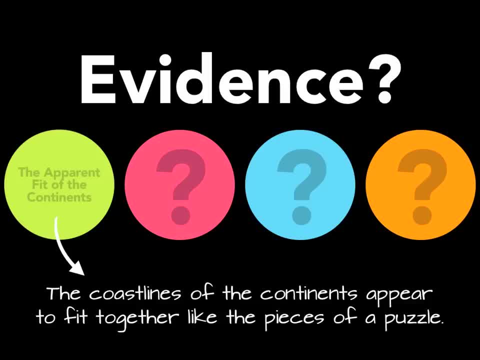 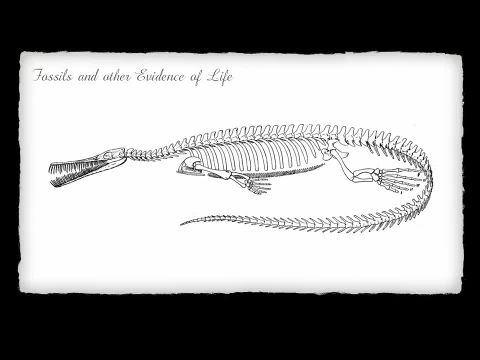 that's not enough. So Wegener went back to the drawing board. He dug through piles of books and libraries and became quite interested in fossils and other evidence of prehistoric life. In fact Wegener became particularly interested in that guy who just swam. 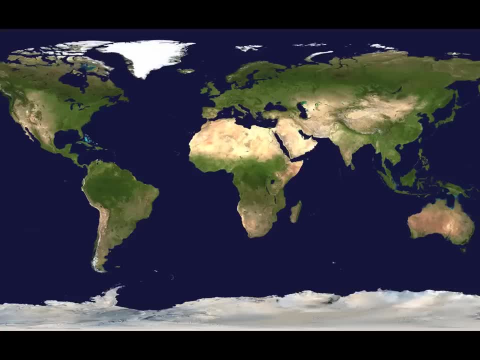 across the screen: the Mesasaurus. Now let me tell you about the Mesasaurus. This is an ancient reptile that lived only in shallow freshwater. What's interesting, though, is that there's only two places in the world where we find fossils. 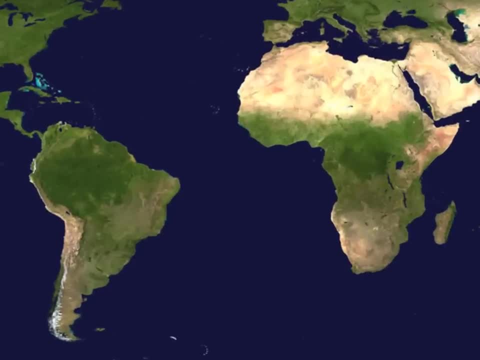 of this freshwater creature. One place is the eastern coast of South America and the other is the western coast of Africa. Now, there's a couple possible solutions for this Now. either the Mesasaurus was living on one of these continents and somehow learned how to fly across the 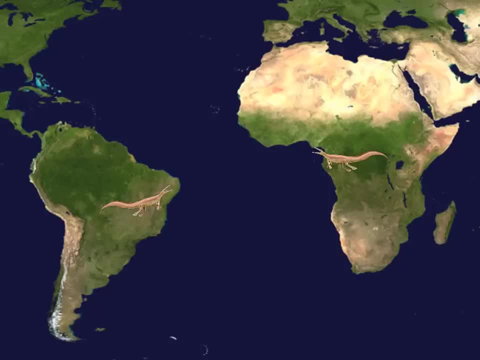 Atlantic Ocean to inhabit the other side of the other continent. But that's not likely. The Mesasaurus certainly could not fly And we know the Mesasaurus couldn't have swam across. The distance is just too great and they can't survive in saltwater, So that's out of the question. 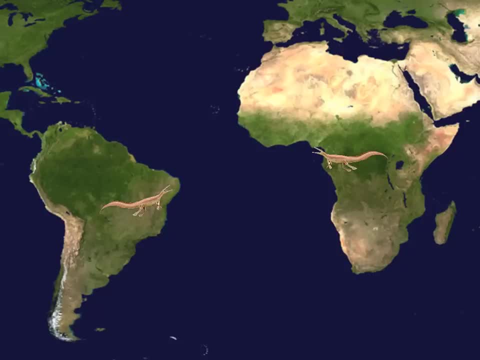 Maybe the water was frozen and he walked across. Well, that's a possibility, but there's really no evidence to support that, And so what Wegener said is that, while the Mesasaurus roamed the land, Africa and South America were connected and they were able to freely walk across. 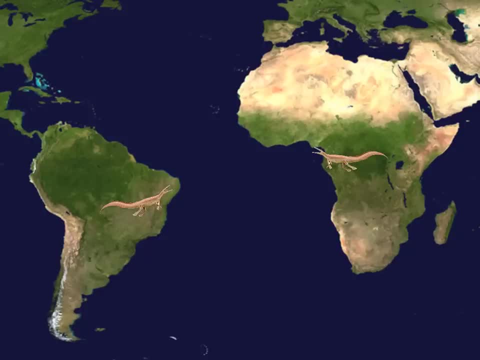 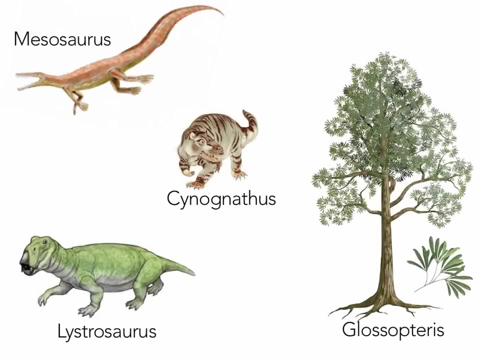 the land masses. And then, after going extinct, the land masses were torn apart and separated, carrying some of the fossils to what would become South America and some to what would become Africa. Interestingly, Wegener looked into this and found that there were other organisms that lived in. 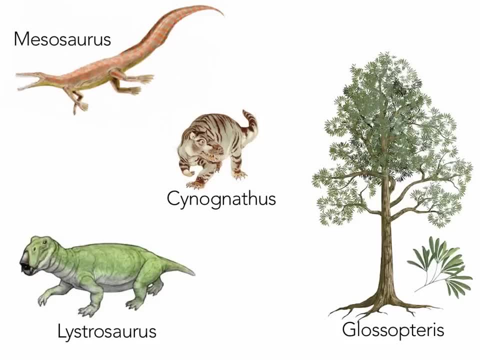 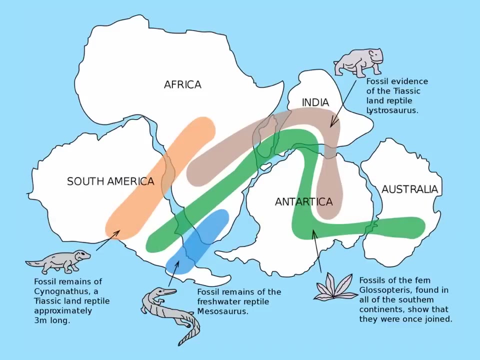 the past that had similar fossil distributions, Cynonathus, Lystrosaurus and Glossoterrus being amongst the more notable ones. These fossils all have these very unique distribution patterns that suggest that the continents were once together And, in fact, if you can reassemble the continents and map out the locations of 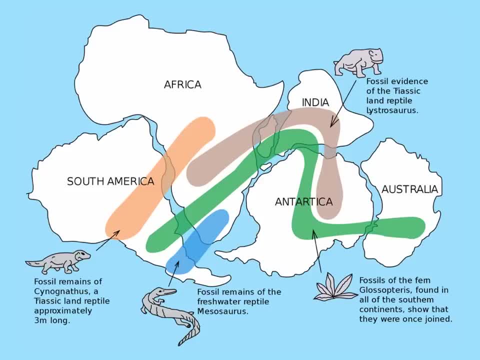 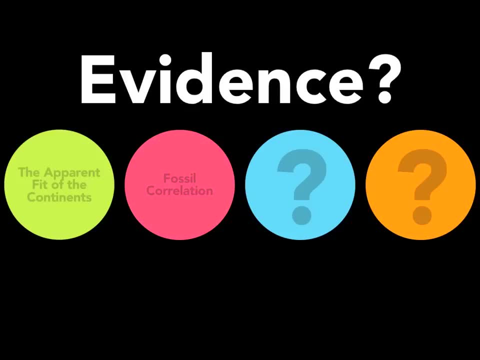 these fossils. they line up perfectly. So that's our evidence number 2.. We call it fossil correlation. Correlation simply means matching up, So matching up fossils on either side of the ocean. To summarize: identical fossils have been found in the rocks. 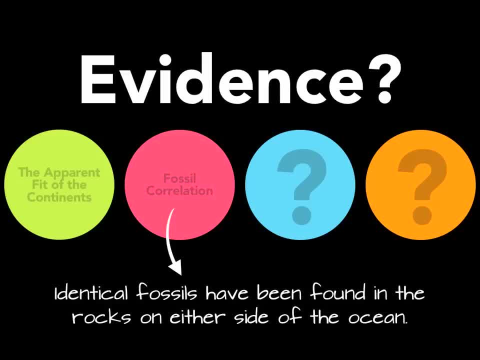 on either side of the ocean, and therefore the continents were once connected and must have been found at different places. The origins of these fossils give us a good idea of how they are linked have drifted apart, But Wegner knew he needed a stronger case, and so he went back to the library. 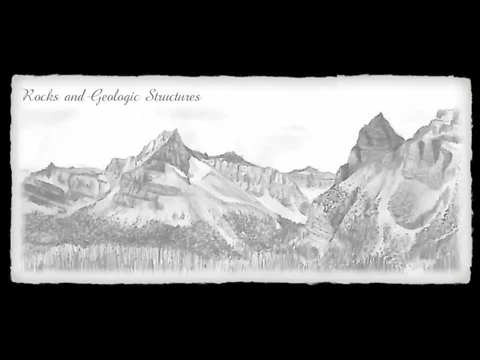 yet again and became fascinated by rocks and geologic structures like mountain ranges of the past, And he found a really interesting pattern, not unlike what he found with fossils. In fact, if we go back to our world map here and let's zoom in on the North Atlantic here, 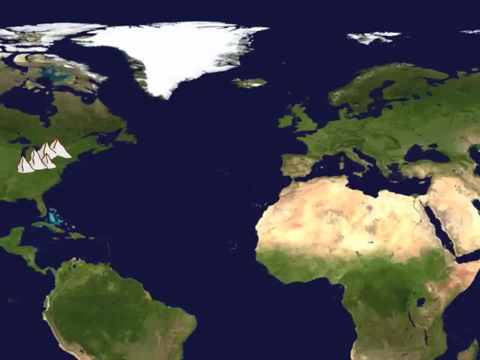 if you look at the mountain ranges in the northeastern United States and the mountain ranges in northern Europe, they match up perfectly, And what I mean is that they are made of the same type of rock and the same age of rock. Now, of course, anything is possible. and the same exact. 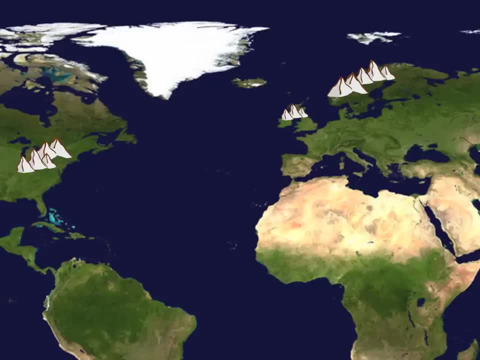 rocks could have formed in two different locations at the same time, But geologically that's unlikely. A better explanation is that these mountains were once connected and as the continents moved they tore them into two, And that becomes evidence number three. We call it rock. 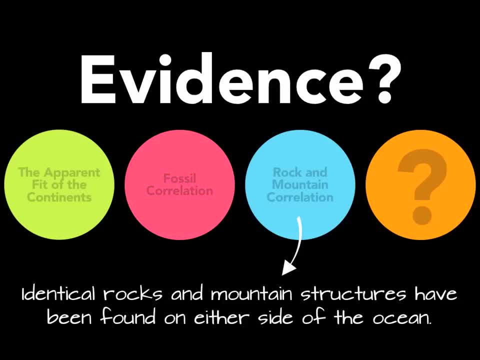 or mountain, And what we see is that identical rocks and mountain structures have been found on either side of the ocean, suggesting that the continents were once connected. But we need one more, and this is probably the most complex of them all. Again, Wegner returned to the library, and this time he 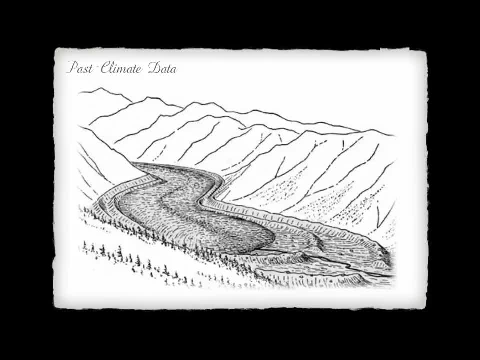 returned to his roots as a meteorologist and he began to look at past climate data, meaning he looked at evidence of cold and warm weather in different parts of the world And he found some interesting evidence. and he found something fascinating. See, he first looked into glaciers, So 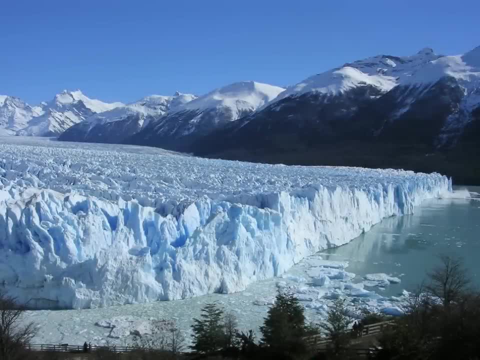 glaciers are these giant rivers of ice that move slowly across the Earth's surface, And, of course, glaciers have to be found in cold parts of the Earth. Today, they're restricted to only the highest mountaintops and, of course, the north and south poles of the Earth. Something interesting. 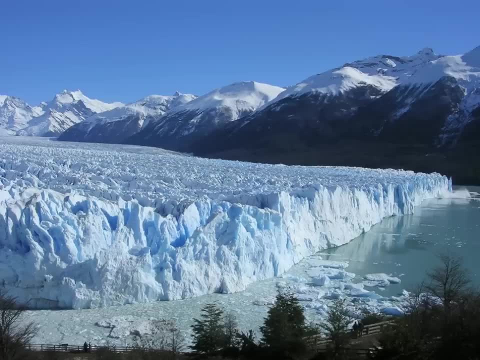 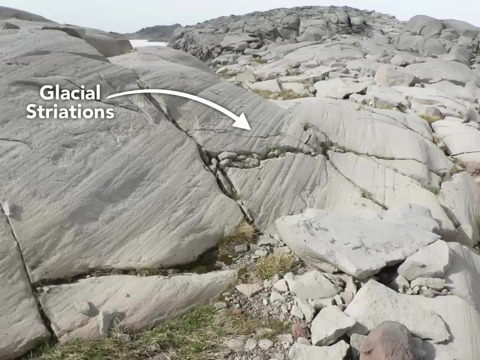 about glaciers is that they move, And when they move over the rock beneath they leave evidence in the form of scratches that we call glacial cracks, And when they move over the rock beneath, they leave evidence in the form of glacial striations, which you see here Now. how does this relate to? 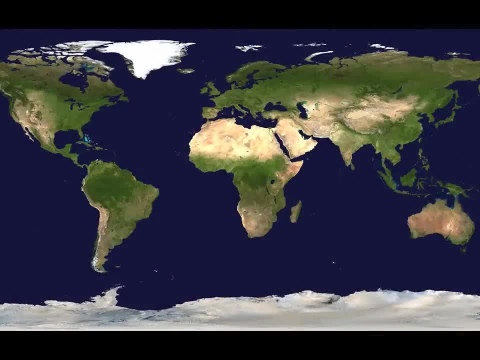 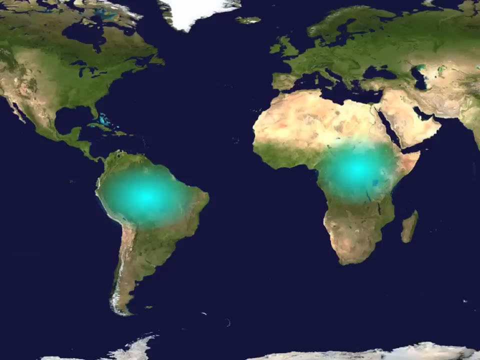 continental drift. Well, if we look at our map, if you look in the present-day tropical rainforests of South America and Africa, you will find glacial striations Here in these two regions. you find these scratches in the bedrock. Now, if you think about that, how could there be glaciers in a 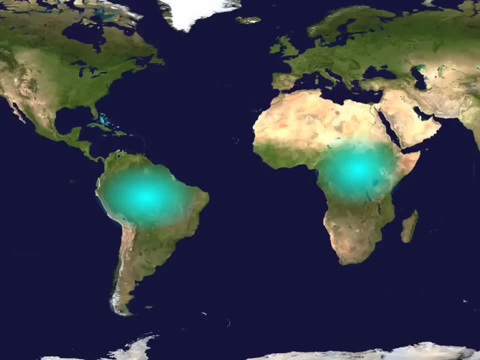 tropical rainforest, unless it wasn't always a tropical rainforest. This suggests that the these continents were not always in their warm equatorial regions like they are now. They were once down near the South Pole where it could have been cold enough to have glaciers, and they have. 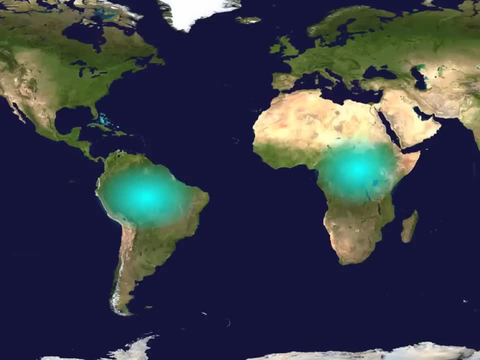 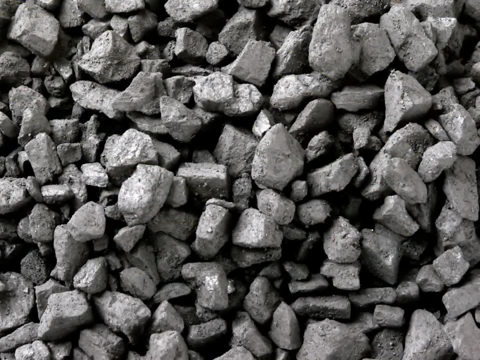 since drifted apart. But Wegener wanted more from this climate data, and so he began to explore a little deeper, And that's when he came across this rock. This is a sedimentary rock called bituminous coal. We know it because we burn it for energy. It's a fossil fuel. 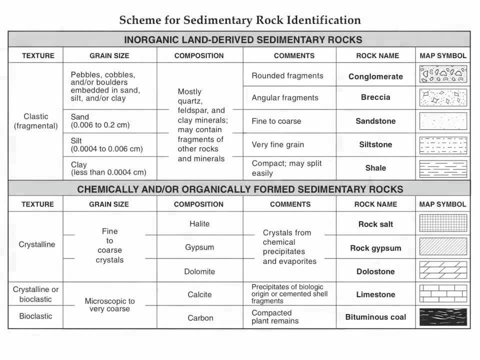 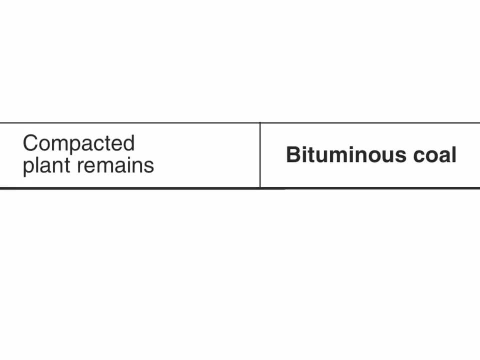 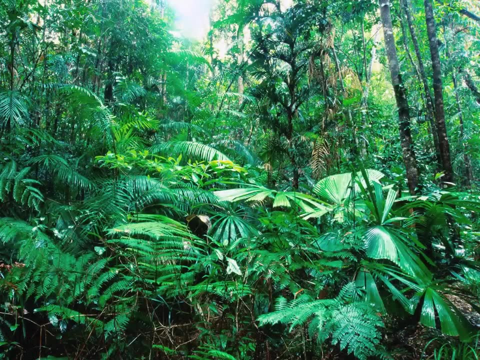 What we know about bituminous coal. if you were to look in an earth science reference tables, you would see that bituminous coal is made from compacted plant remains. So picture tropical plants like this dying on this forest floor and getting compressed over millions of years to form coal. Now let's look at where coal is.